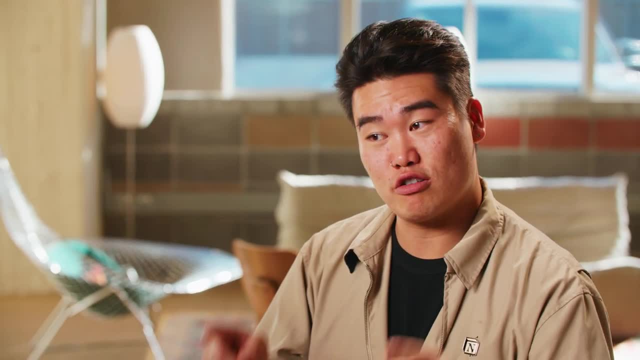 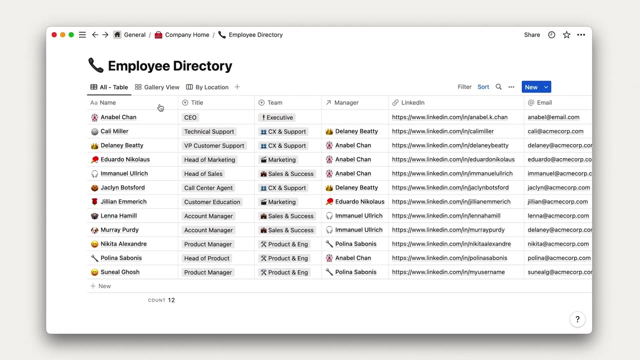 Over the next couple of videos we'll take a tour of databases in Notion and explore that power, Starting with the name property. this property is an identifier for each database entry. It's pretty similar to a page title and describes what you expect to find in that row. 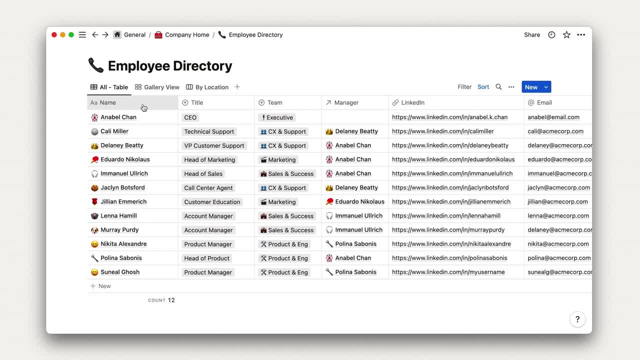 So in our example, every row is a row with a name. Every row is a person that works at Acme Inc. a pretty natural identifier. One pro tip about the name property: it is the only property in a database that Notion requires you to have. 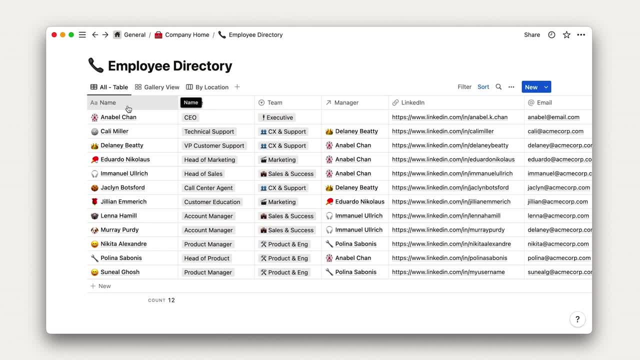 Others can be deleted or their type modified. This will be good to know as you start to build your own databases. After each name we see columns with descriptions of the person. These columns are also called properties. You'll hear me use the terms interchangeably. 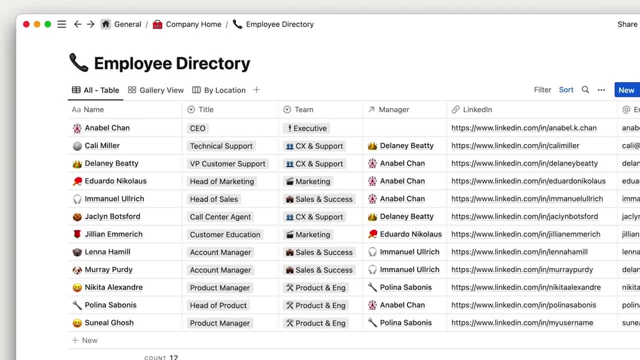 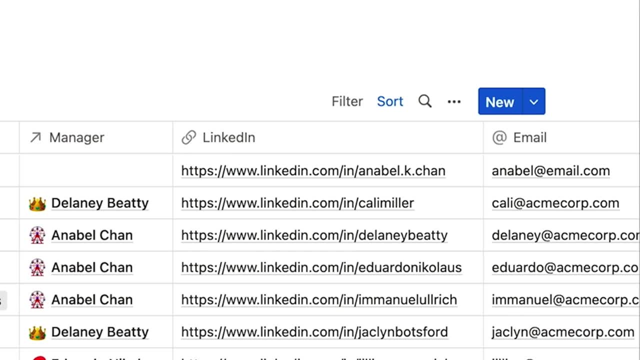 Here you can see a number of different properties. Here you can see a number of different properties. here you can see a number of different properties that describe the person, like their title, team manager, LinkedIn profile, email and more. 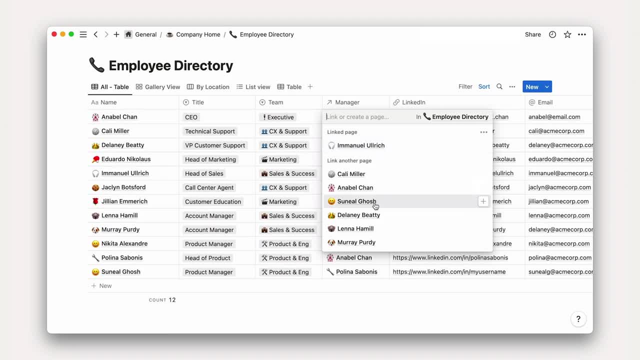 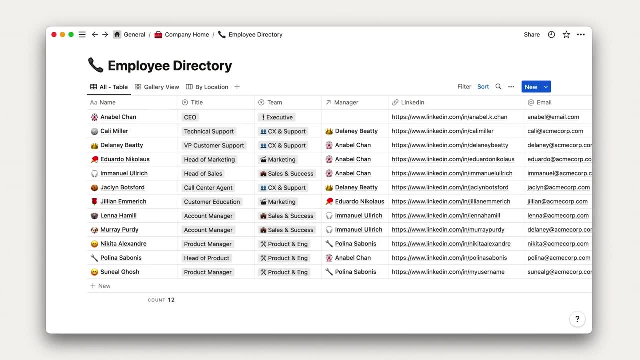 You might also notice that these columns look richer than your traditional spreadsheet with formatting, color and interactivity. Unlike a spreadsheet Notion, databases require each column to have a type, literally a data type, which you can sort of think of like block types. 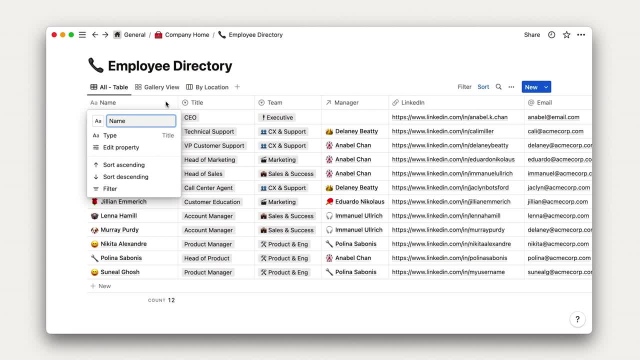 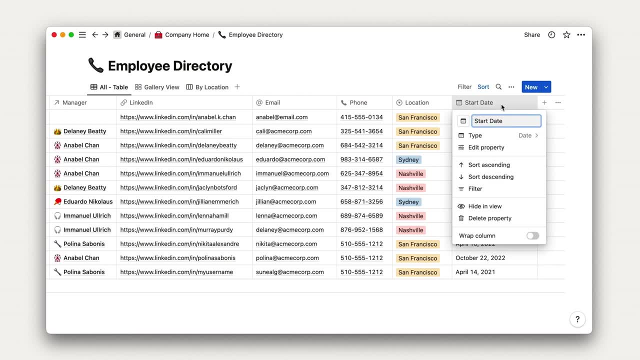 For example, for example, this name is a block type. For example, for example, this name column is a special name type. The team and location columns are tags, The start date is a date And the LinkedIn profile is a URL. 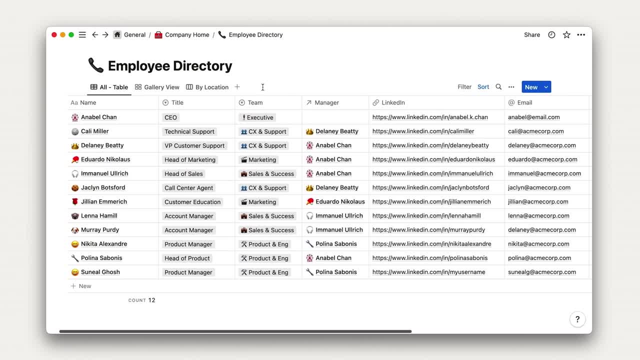 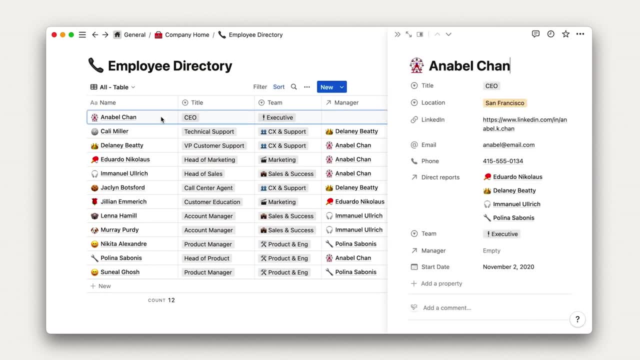 This means that they can be uniquely formatted and displayed in different layouts, which we'll get into soon. The last thing that I want to show here is that each row in a database actually opens up to its own page. Literally everything that we've learned up to this point can be used inside of a database. 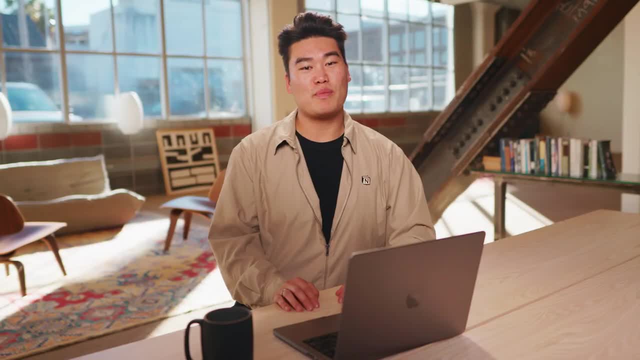 Literally everything that we've learned up to this point can be used inside of a database. Literally everything that we've learned up to this point can be used inside of a database. Moving on from the tour, let's go ahead and create our own database in Notion. 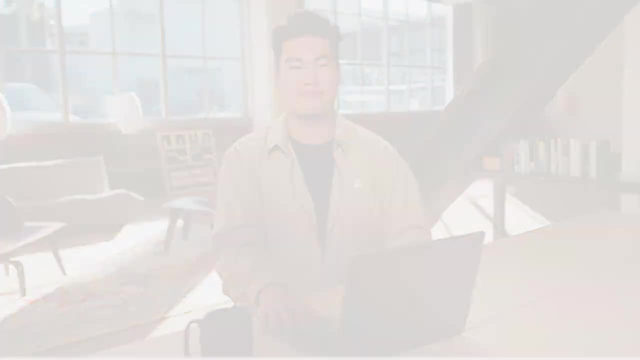 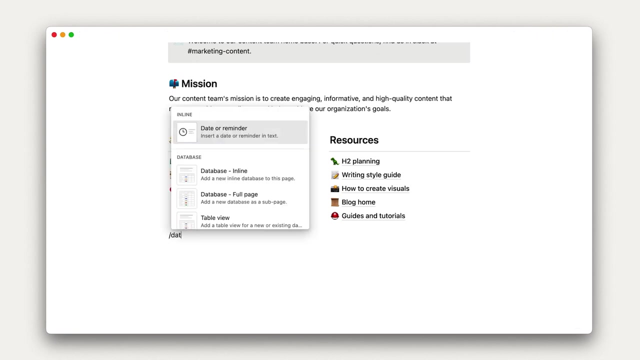 We'll build out the framework of a content calendar for a marketing team. We'll build out the framework of a content calendar for a marketing team Just like any other block type. in Notion, a database can be added with the slash command or the plus sign.